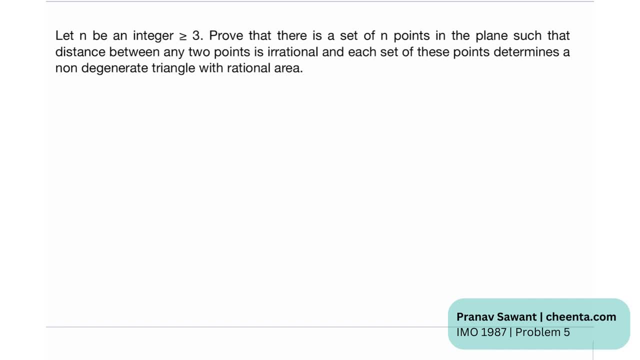 determines a non-degenerate triangle with rational area now. so this might seem very worthy to you it's- and i agree it is unnecessarily worthy to a particular extent. but uh, really, what they're trying to say is that you have a triangle, you have a triangle, you have a non-degenerate. 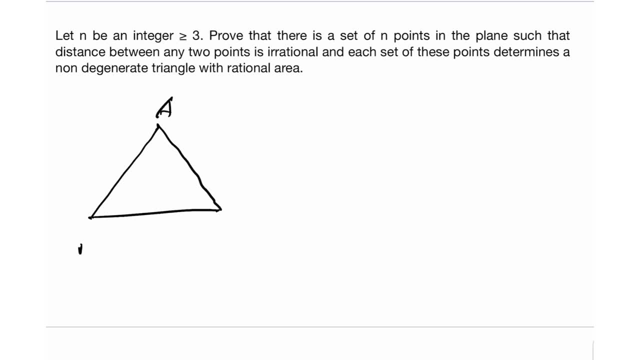 triangle, such that the side of the triangle is a non-degenerate triangle and the side of the triangle, if i label that as a, b, c, the side lengths a, b, b, c and a, c are irrational. if i'll represent that as q bar and the area of this triangle, a, b, c, this is actually a rational quantity. that is all that. 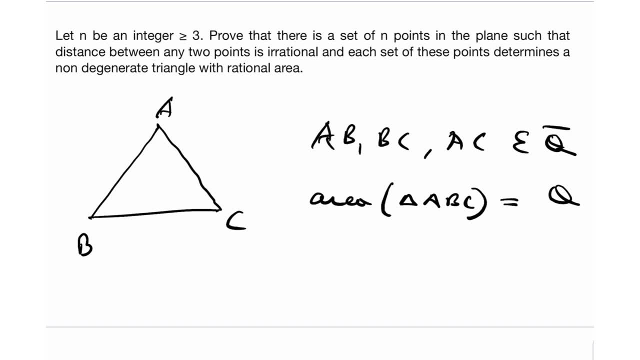 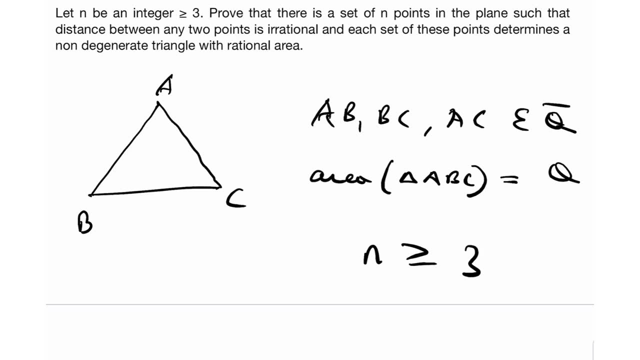 they're trying to say, and we need to prove that this exists for um, any end points in the euclidean plane right and n is obviously greater than or equal to three. i mean obviously, because you cannot form a triangle with only one or two points right, so n has to be greater than three, of course. 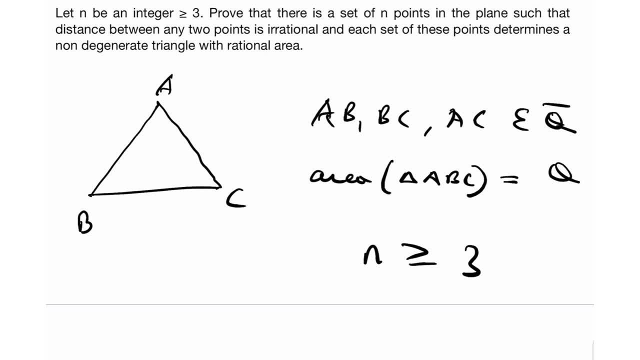 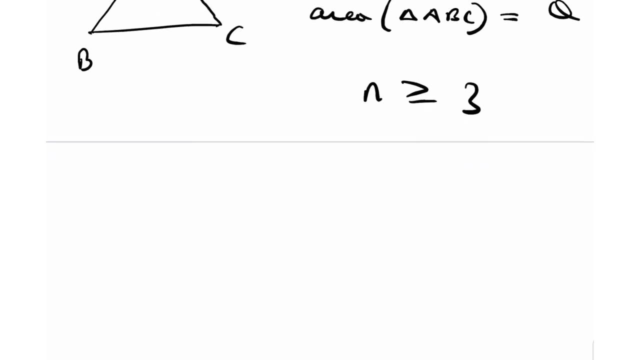 so, at the end of the day, the core idea of what we need to prove is that, even though sides are irrational, the area can still be rational, so prove the existence of that claim in a way right. so before we really get into this problem, i want to introduce you to something called as lattice. 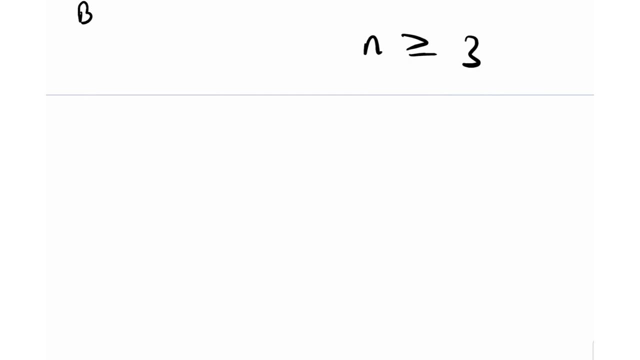 points. now, really, lattice point is nothing but a definition. so lattice points is any point on the coordinate axis. so let's say this is a coordinate axis- x, y, and then we have any point, p. let's say x. so p will be a lattice point if both x and y are integers. x is an integer, y is an integer. 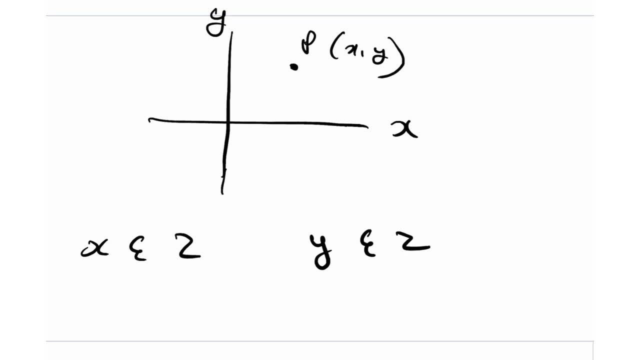 and if both its coordinates are integers, it's a lattice point. it's as simple as that. it's really as simple as that. both coordinates are integers. there you go. it's a lattice point. right as simple as that. so lattice, in a way, is just representing the word integer. right as simple as that. now for 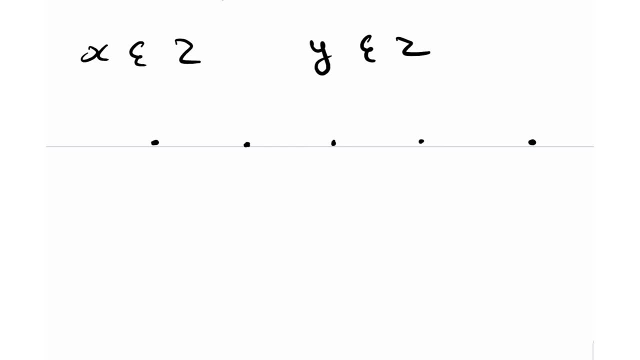 example: one, two, three, four, five. let me just draw this grid, and each point that i'm marking represent this point, right? so it represents some lattice point. let me just draw maybe a couple of more lines and then we are good to go. so here i'm just going to draw a triangle, so let me just take any. 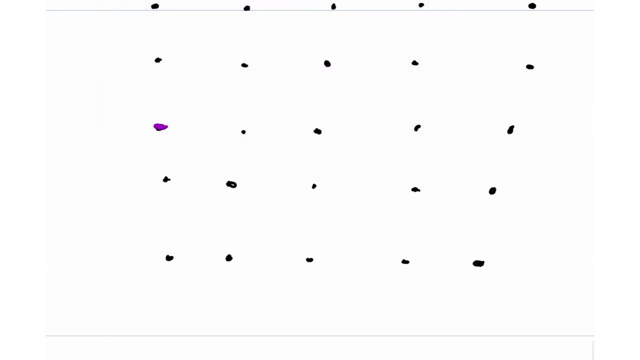 three points, really, and make a triangle. right. let's take this point, let's take- i don't know- this point and maybe this point, and let's just make a triangle by, you know, joining these three points. okay, awesome, right? so now you've, this triangle is actually a lattice triangle, right, because all of its three vertices- a, b and c. 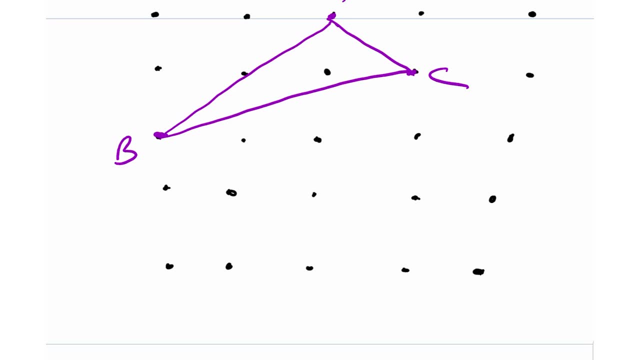 are lattice points. right, all of these three vertices, the coordinates of these three vertices are integers and therefore it's a lattice point. this should remind you. a point p will be a lattice point if x comma y will both be integers. so, for example, 1 comma 1 is a lattice point, you know 7. 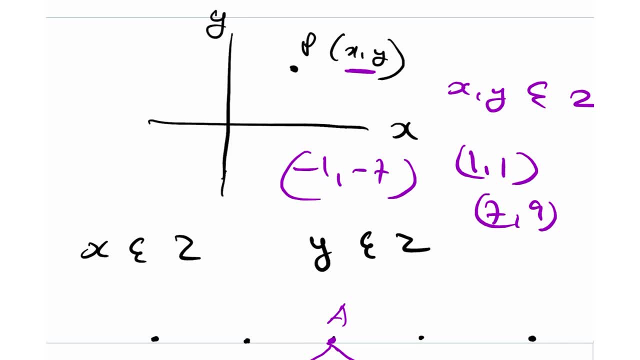 comma 9 is a lattice point. negative 1 comma negative 7 is also a lattice point. any integer really, but something like 1 by 2 and 7. this is not a lattice point because 1 by 2 is not an integer. it's really as simple as that. 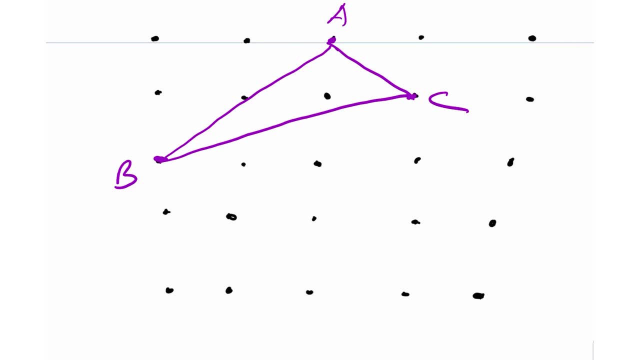 so over here on this grid, you can clearly see that a, b and c are all lattice points, so all are integer points and you can just consider this as one unit. but really those that's unnecessary, but okay. so yeah, all of these three points are lattice points really. but now, what i can, what i. 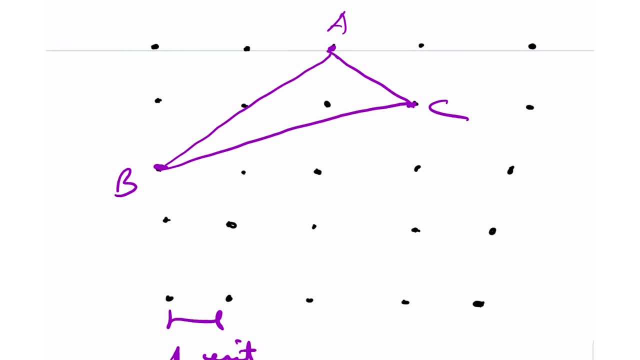 want to demonstrate to you is because these three are lattice points, the area will be rational. so, in a way, the claim that i'm making is: if you have a triangle, any triangle, any triangle, any triangle- a, b, c- such that a, b and c are lattice points, then the area of this triangle will be rational. right, it will be rational. this is the 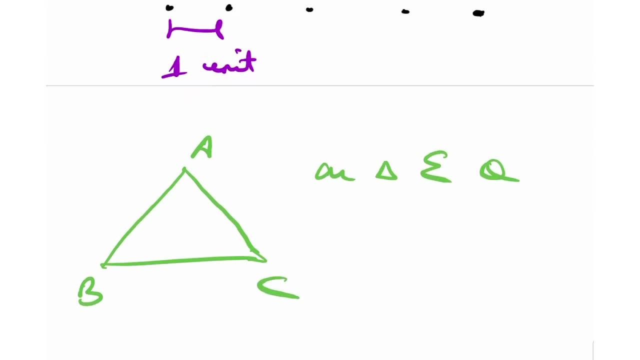 claim that i'm trying to make, and i'll prove this in a couple of ways. right, just to remind you again. what i'm saying is that if the points a, b and c- all are lattice points, they have coordinates as integers. that means that the area of that triangle, any general 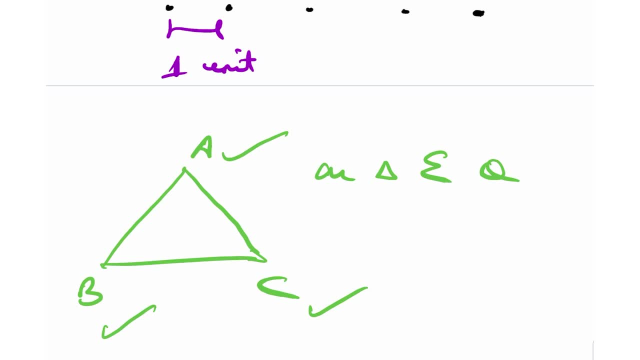 triangle that has a, b and c as lattice points will be rational quantity. there are a couple of ways to prove that. first would be geometrically. you know, that's why i made this diagram, otherwise i could have proved- just given you a theorem and proven it right. so if i just draw a minimal 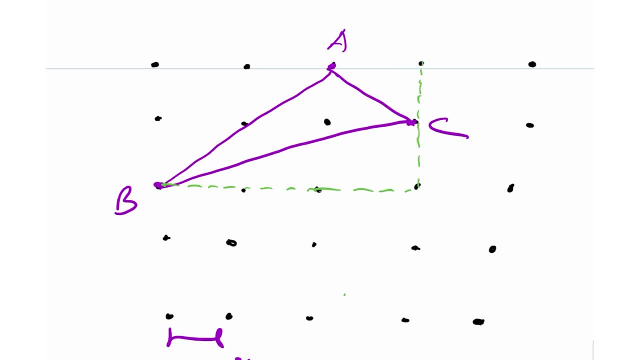 rectangle enclosing this triangle. so this will obviously be the smallest rectangle, smallest, mind you, that encloses this. you can take a larger one also, but why too complicated? you know this works perfectly as well. now, the area of this rectangle will obviously be rational. you can find the 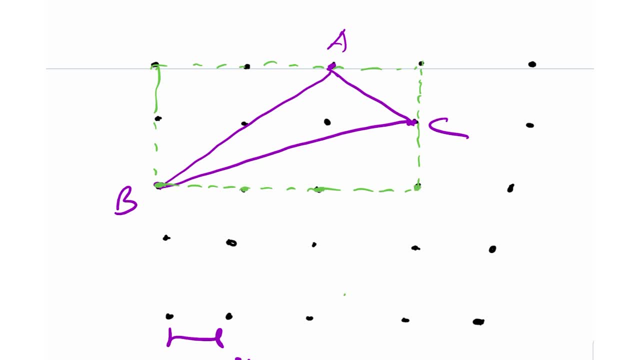 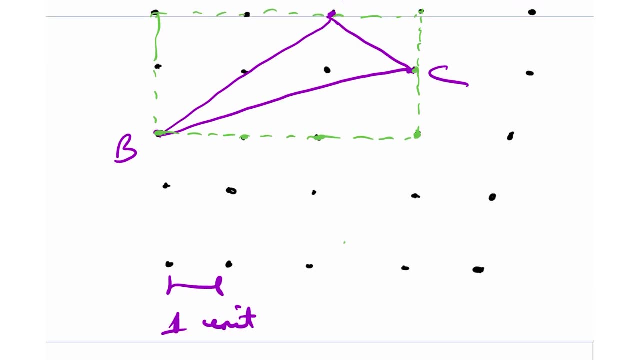 point. it also right, it's. you have how many points? one, two, three, four. so the length is four. and what's the width? you have this first point, you have the second point, this is third point. so width is three. like i said, this is one box. one. one is one unit, so the area is 12. well, area is an integer, it's. 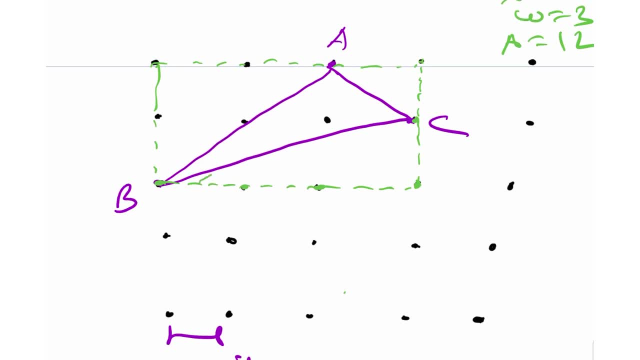 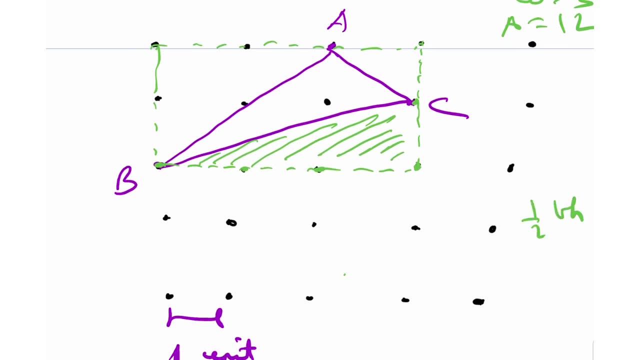 obviously a rational quantity. but now you see that the area of this triangle that i'm shading is also a rational quantity. why? because it's half into base, into height. so no matter what the base and height are, well, base is one, two, three, four, base is four and height is one. so area is obviously two. 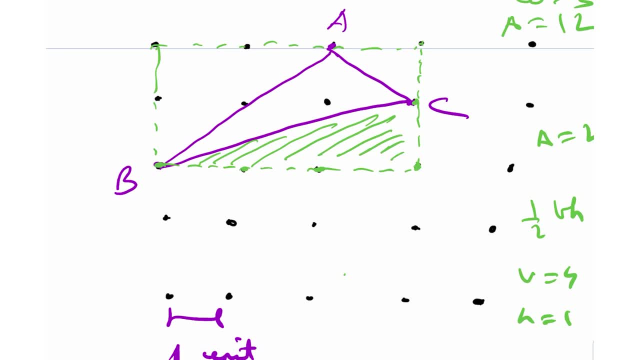 but it doesn't matter, these are just values. the core thing is that it is rational. similarly, this area, this area is also rational quantity. it is going to be half into one into one. it is 0.5. it is rational one by two. similarly, this area is also going to be rational quantity, you know, because half 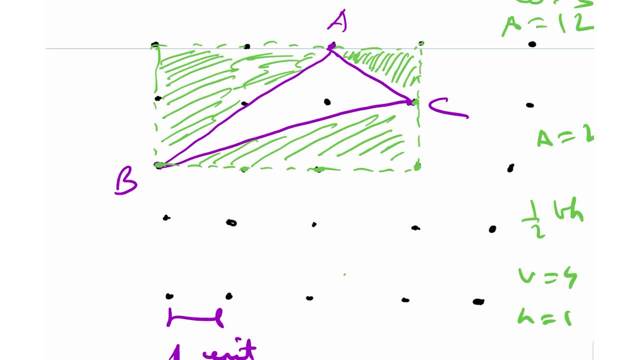 into base, into height. base and height are both integers divided by two. at the very least, you're getting a rational number, if not an integer, if not a natural number, right? so that means, if these three shaded regions that i've shaded in green, you can get a rational number, if not a natural number. 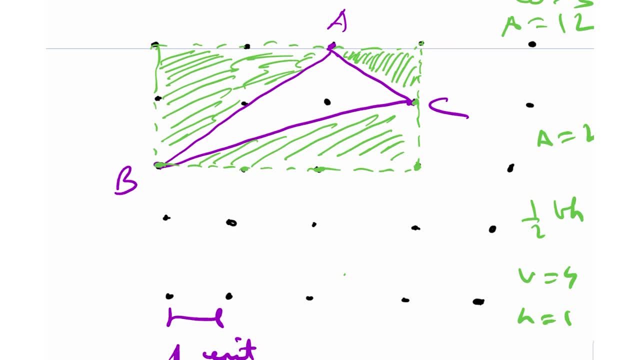 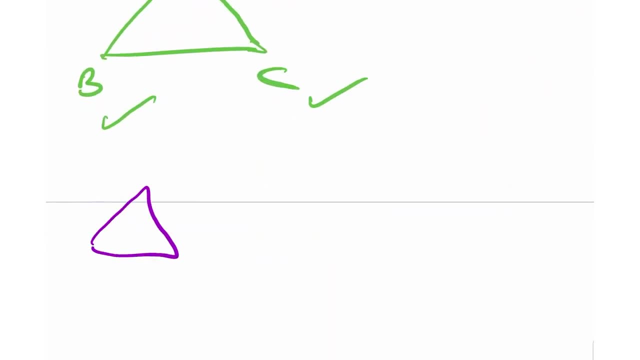 and the entire rectangle is also a rational quantity. that means this is also has to be a rational quantity, right, because effectively the area of this of the purple triangle, area of the purple triangle, is nothing but area of the rectangle. i'm just using shading notations over here, i hope you don't mind. minus area of all the triangles shaded in green right we have. 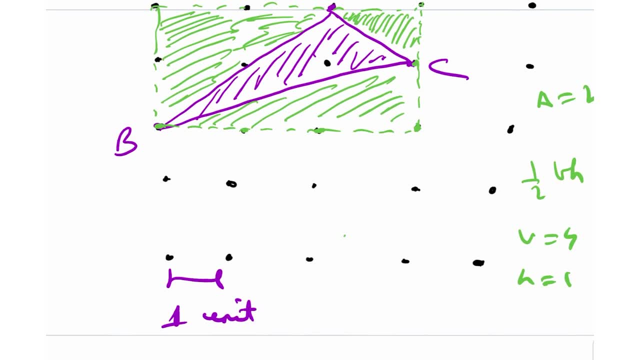 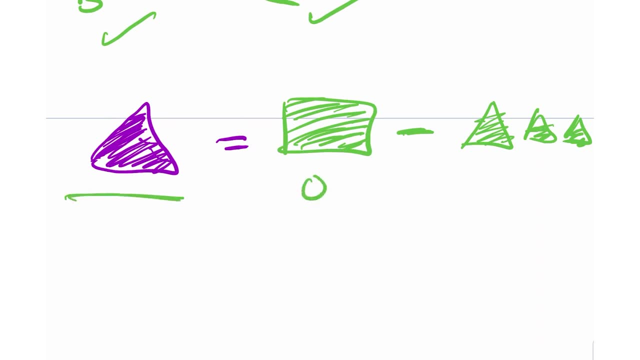 three triangles. i'll represent it as like this: right, three triangles: number one, number two and number three right. so the area of this, uh, purple triangle is going to be area of the rectangle, which is the rational minus the sum of the areas of these three triangles and, obviously, 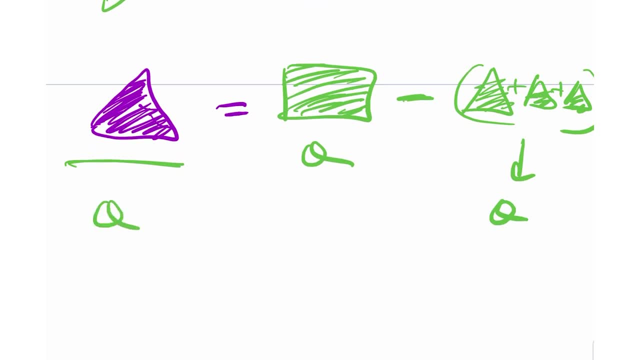 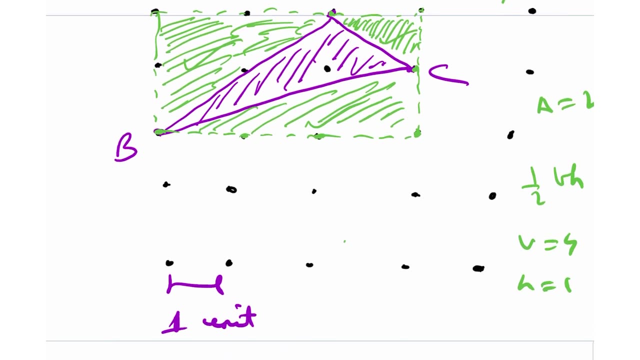 all of these three will be rational as well, so automatically this becomes rational quantity as well. so that is essentially proving my claim right. my claim was that if all three points- a, b and c- are lattice points, that means the area is rational. and we saw with this geometrical interpretation as 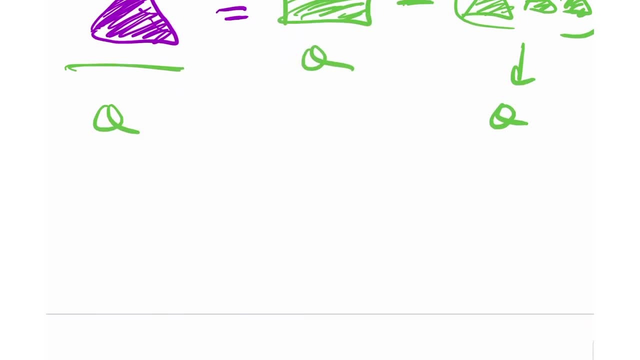 well, now there's another way to really see this, and that is where something called a spick's theorem- you know pick's theorem, pick's formula, you know you can say anything. really. pick's theorem says that the area of a lattice polygon is equal to i plus b by 2 minus 1, right where i is the number. 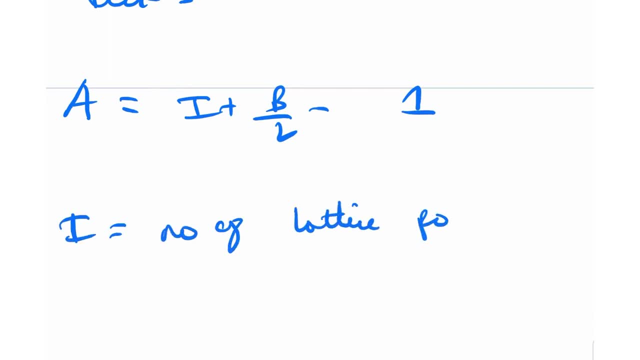 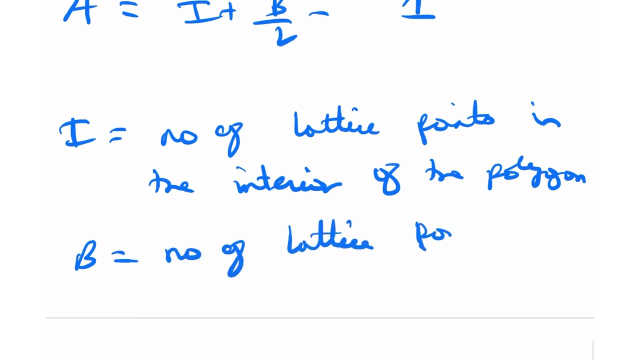 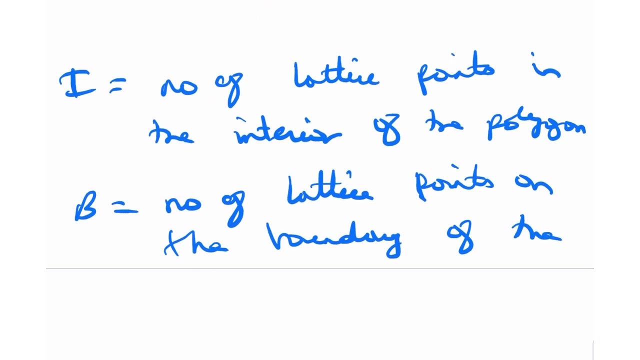 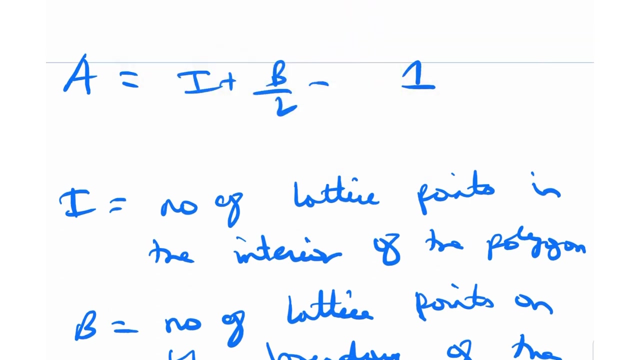 of lattice points in interior or in the interior of the polygon right, and this b is the number of lattice points on the boundary, on the surface, on the boundary right of the polygon, of the lattice polygon, and a is obviously area of such a lattice polygon. now you clearly see that i is number of. 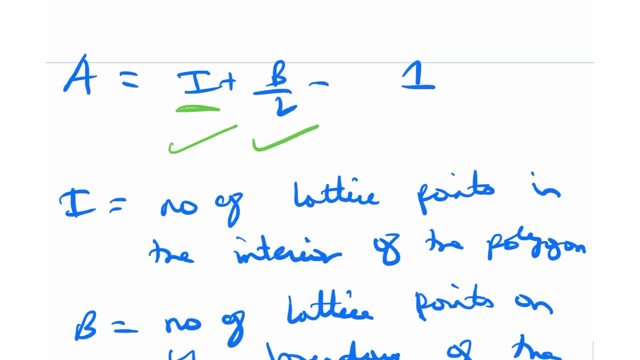 lattice points. it has to be natural number. so this is rational. b by 2 will be rational. one is rational. you combine all of these three together. area becomes rational. you know this. this is just 10. second analysis. uh, easily provable. i is rational. b by 2 rational. 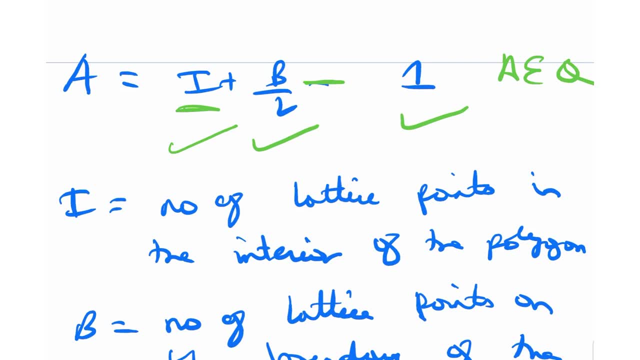 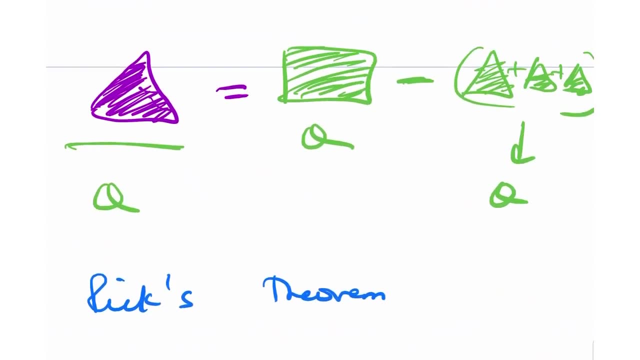 one rational, add two, subtract one, you get a rational quantity. so area will be rational right and a lattice polygon, essentially polygon, that has all its vertices as lattice points. so, like i said over here, this triangle that i made in this figure over here also has lattice points. 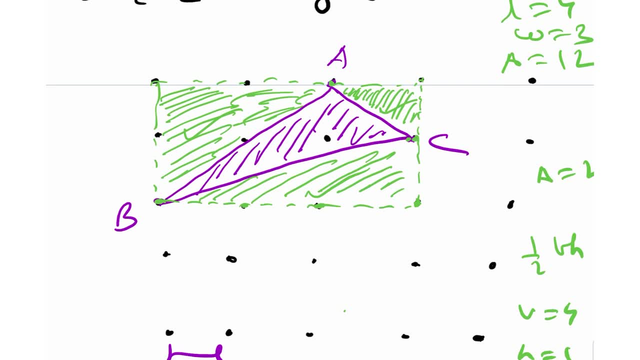 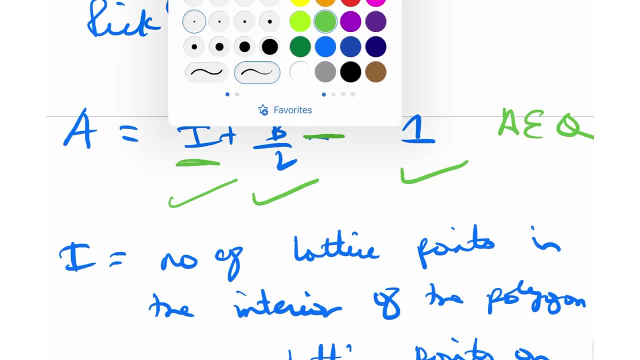 it is a lattice polygon, as it as its vertices are all lattice points and hence its area will be rational, which we can see from pick's theorem as well. so really, uh, there are multiple ways to prove this. now, how is this related to a problem? now in the problem, 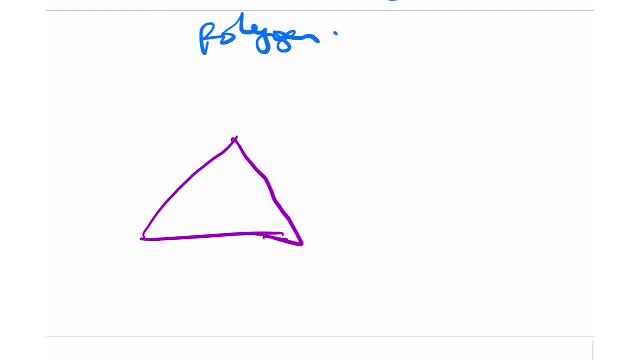 if you remember in the problem, if you remember, they said that the area is rational. so if the area is rational, that means the points, the points on triangle con. they correspond to lattice points, right, if i call that as? let's say, x, y and z, x, y and z, all are lattice points, because whenever we 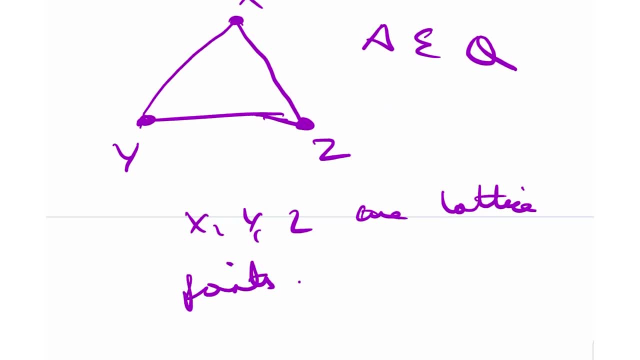 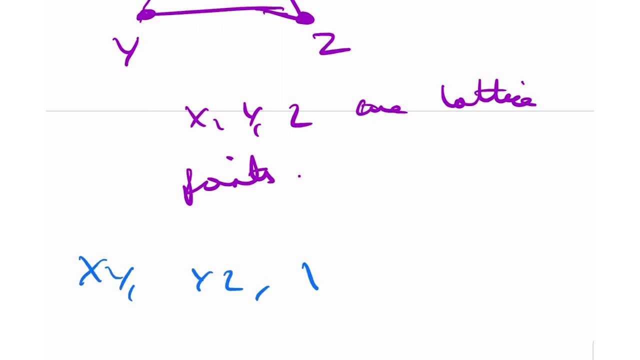 have lattice points, the area will be rational. so we have satisfied the condition for area to be rational just by considering lattice points. it was as simple as that. you consider lattice points, you consider the area as rational. but we need to also consider the fact that the side lengths x, y, y, z, x, z. 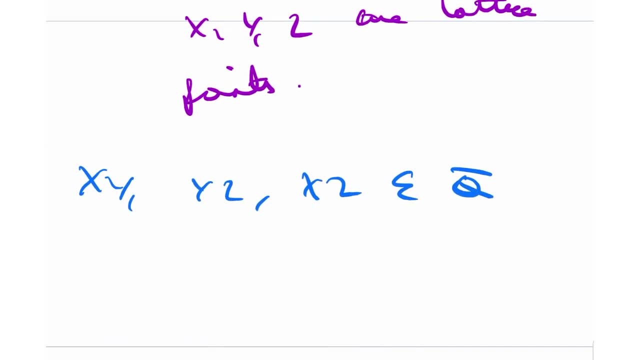 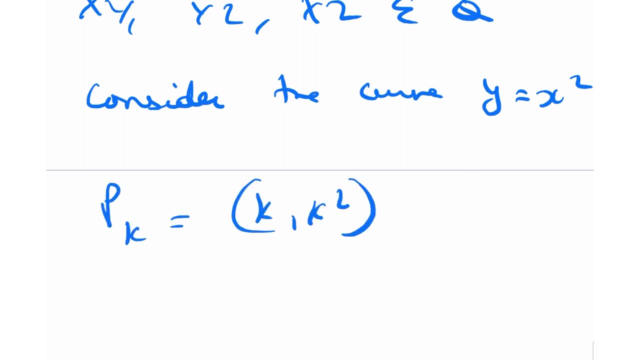 needs to be irrational right and to see that i'm going to consider a curve. consider the curve: y is equal to x squared right and i can define any point- p, k on the curve to be equal to k, comma, k square right, where k runs from one, two, three, all the way up to n, because we have 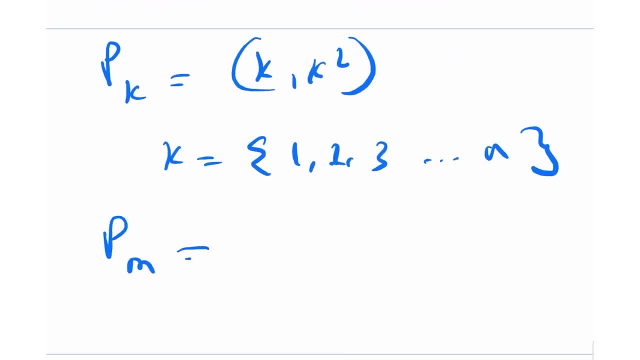 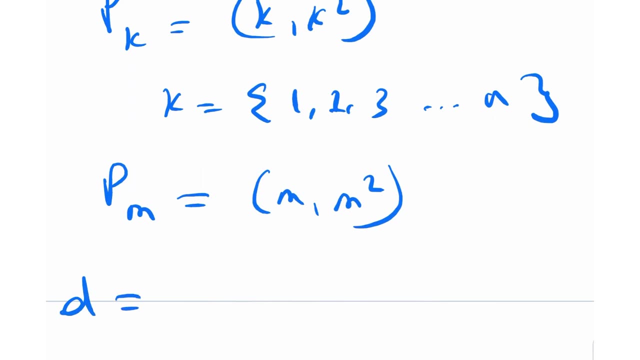 the same, right, okay, great, now again i can define a point, p, m, as m comma, m square, and obviously both these points lie on the parabola. now, if i define the distance between these two points, it would be nothing but square root of k minus m whole squared, plus k squared minus m squared whole square this: 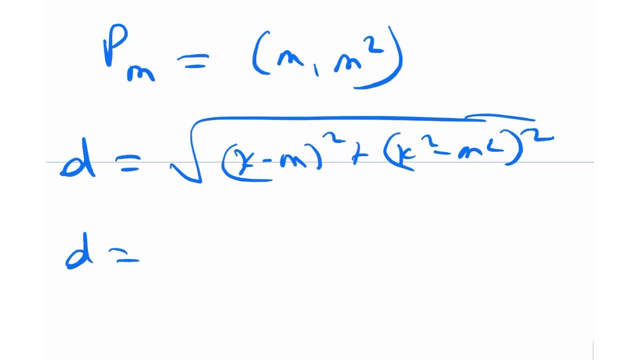 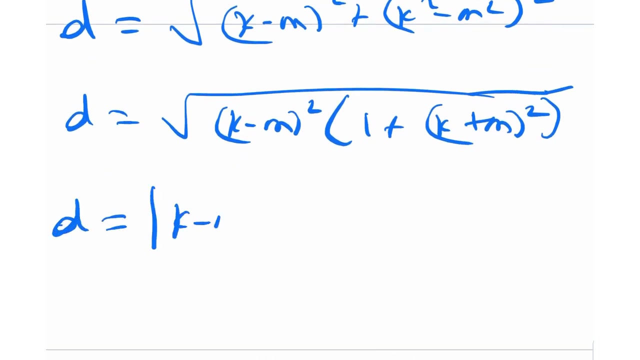 is very trivial from distance formula. so d becomes: i can take k minus m whole square common over here. i'll get one plus um, k plus m whole square over here, right, i hope i'm doing this right. so i'm going to do it correctly. yeah, looks good. so i can take this modulus of k minus m out. remember square root of. 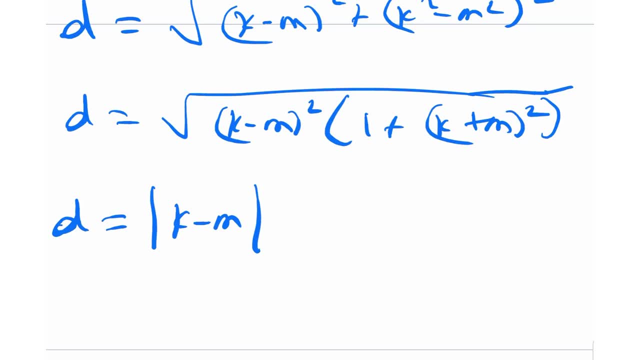 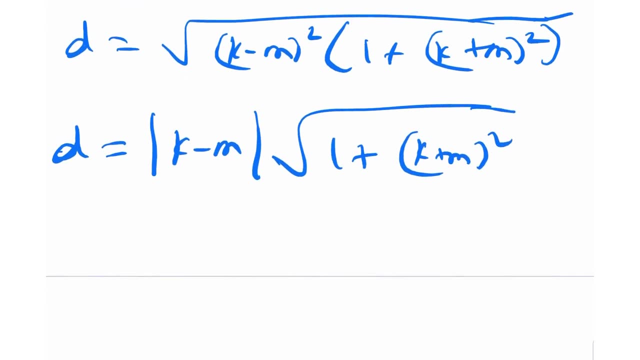 x square is modulus x. right square root of x square is not x, it is modulus x, don't forget that. and then you have in the root one plus k plus m whole square. now, really, this quantity over here will always be irrational. right, it will always be a radical, because square root of a square plus b. 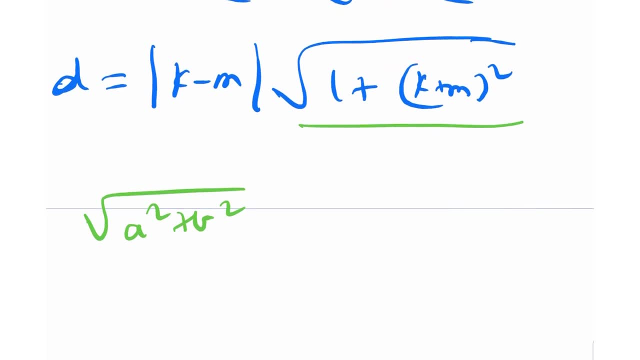 square is always a radical quantity. it's always an irrational quantity until unless a and b are both zero. clearly, we have one over here, and this is also non-zero quantity, so d is irrational. do you actually see what i've done here? well, if this algebraic thing does not make much sense to you, 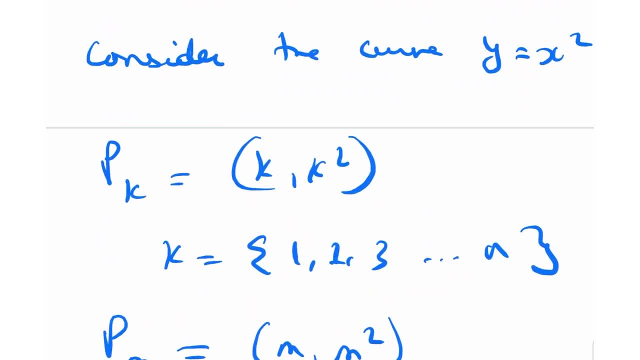 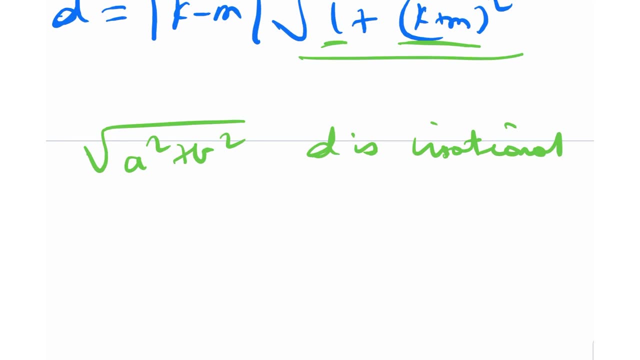 this seems very arbitrary, that pranavi just considered a curve and just did some random calculations and it made no sense. i mean, it did make sense algebraically, but what's the geometrical interpretation? how this connected to the question. well to know that. let's just graph. 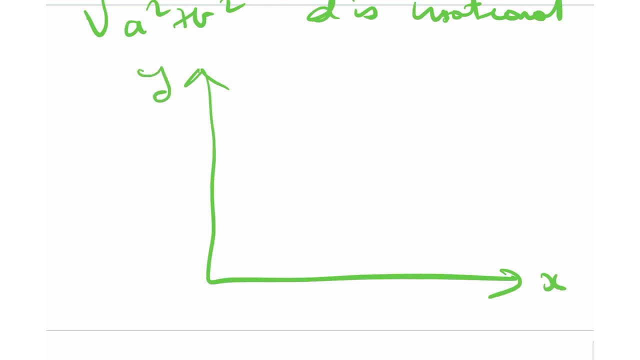 it out. so this is our x-axis, this is our y-axis and this is our curve. y is equal to x square. now take any three points on this curve. let's say one comma one, let's say two comma four, let's say three comma nine, and construct a triangle using these three coordinates. 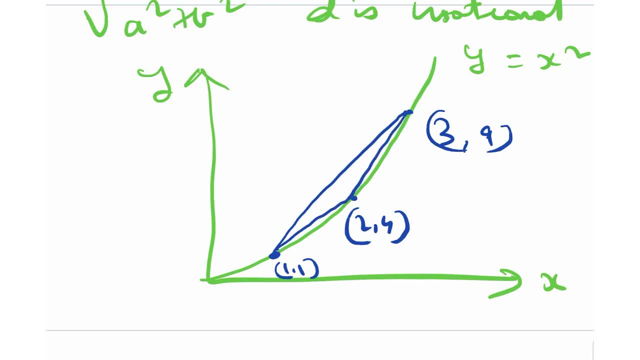 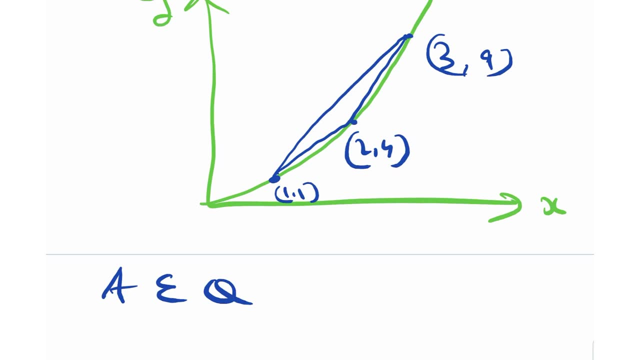 there we go. that's a triangle. now will this triangle have rational area? yes, all three points are lattice points. area will be. area will be a rational quantity. we've seen that as well. and all of these distances- if i just label this as a, b and c- a, b, b, c and a: c- will be irrational. 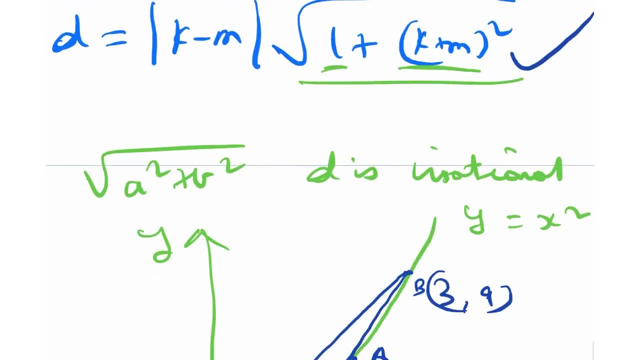 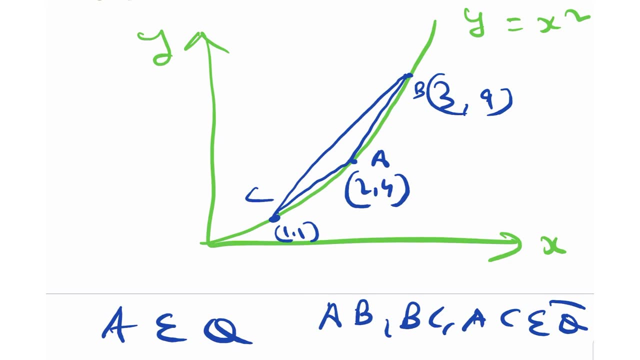 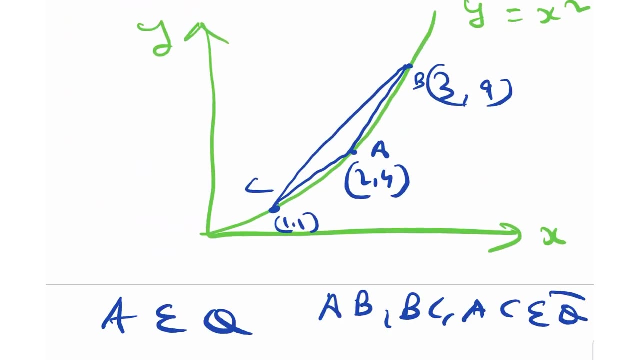 this is what i'd proven over here, right? if we consider a, y is equal to x square, this parabola, really distance between any two points- is irrational. i proved that for any two general points, right. i took k and m to be any variables, random variables, and from there we essentially 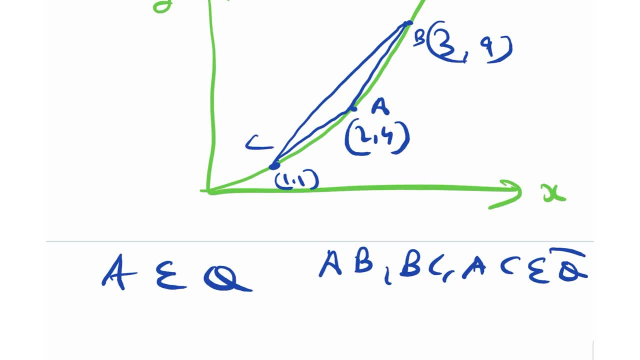 saw that distance between any two points is irrational. that is proving our question and in fact we have proven our question. so we have found a triangle such that its side lengths are all irrational but its area is rational right, and because there are n points on this curve, 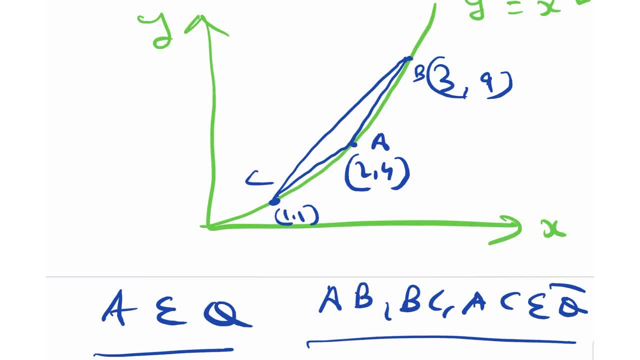 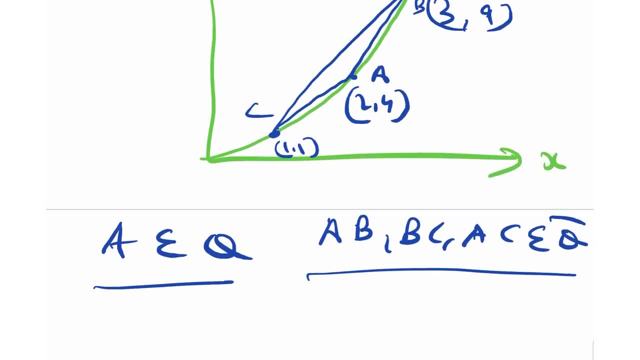 you can form a series of n, c, 3 degenerate triangles, and hence we have proved what we had to prove in the question right. so quite a fascinating question, and really the only idea was that, as long as the vertices are lattice points, the area will, by definition, be rational from pick's theorem. and then we consider this curve and we can get the same thing with the other vertices. so we can get the same thing with the other vertices, and we can get the same thing with the other vertices, and we can get the same thing with. 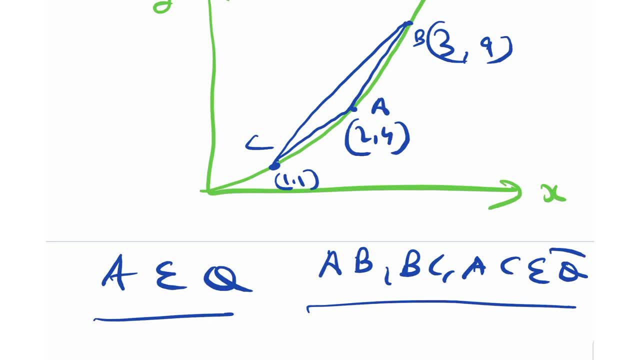 the other vertices and we can get the same thing with the other vertices и bands. the same thing again. kidding, by the way. so here i've gone through thevisible. for instance, here we had, x is equal to 1 and the second is 1 x that's also equal to one. so we have. 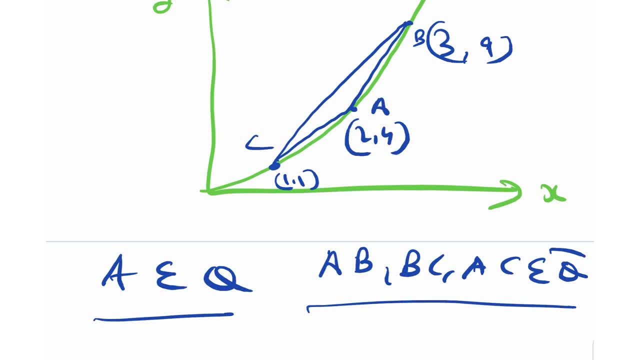 the similar formula, which means that here the path along which you are considering for what is coupled over and part down is equal to 0 and the only result used is a 0.. 2 eh. 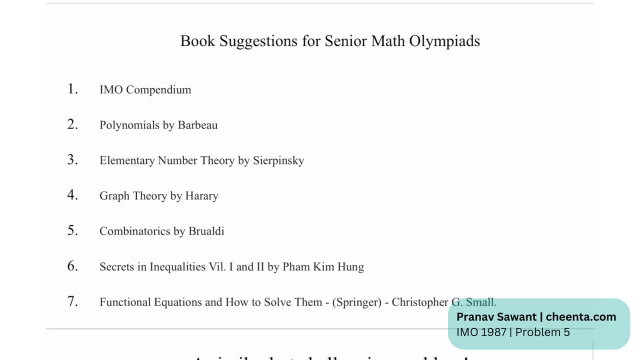 of senior math Olympians: Amok Compendium. Polynomials by Barbeiu, Elementary number 3 by CF Pinsky. Graph Theory by Harari. Combinatics by Broualdi, Secrets and Inequalities and Functional.